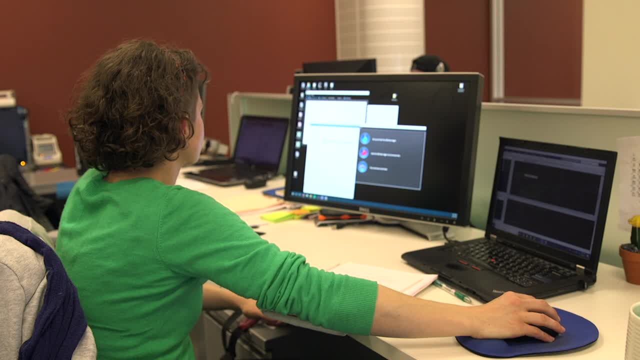 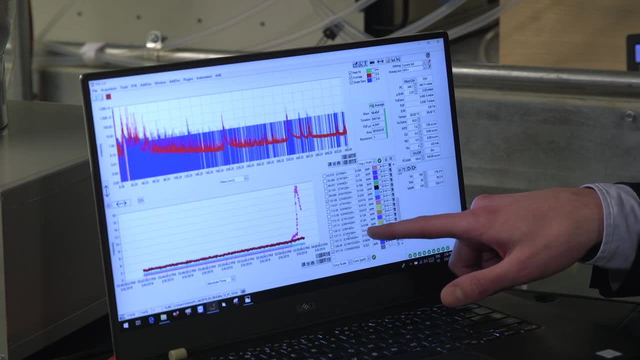 through their exhaled breath. also the personal care products that they wear on their bodies, such as deodorant, as well as building materials and furnishings. We just saw a huge spike in the concentration of monoterpenes. They're associated with with the odor of orange or lime or lemon. 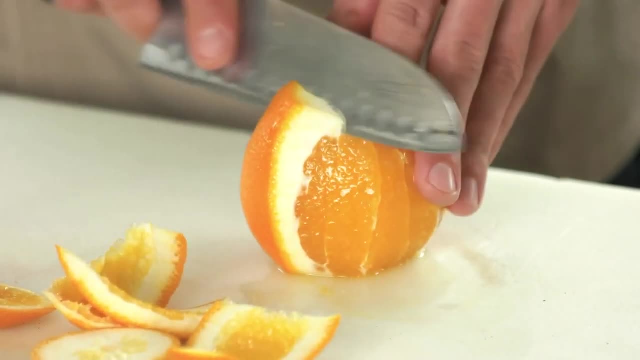 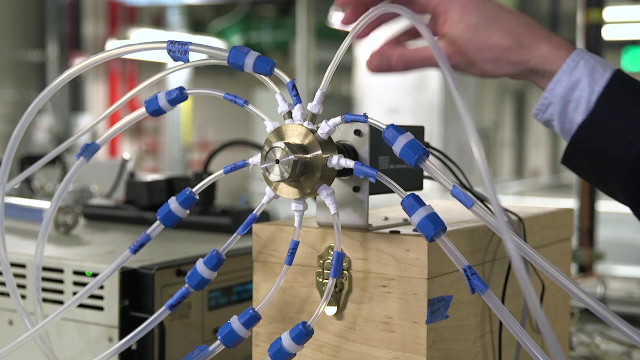 Likely somebody peeled an orange or a mandarin in the common area outside of the office. So this valve system allows us to track how the concentrations vary in space. Each of these teflon tubes go to different sampling locations in the ventilation system, and then we switch. 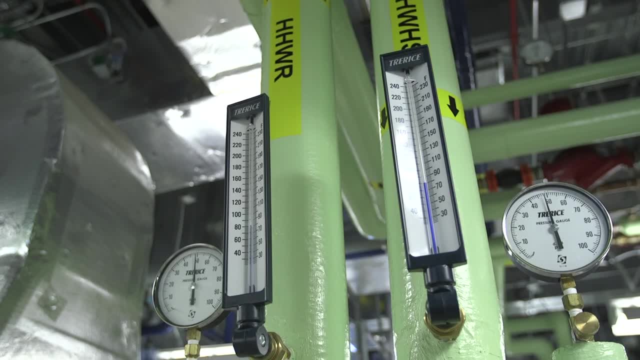 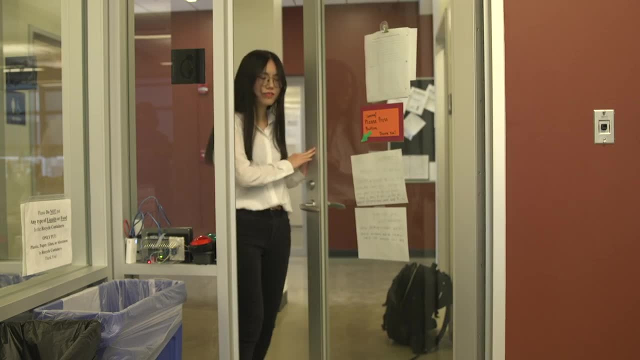 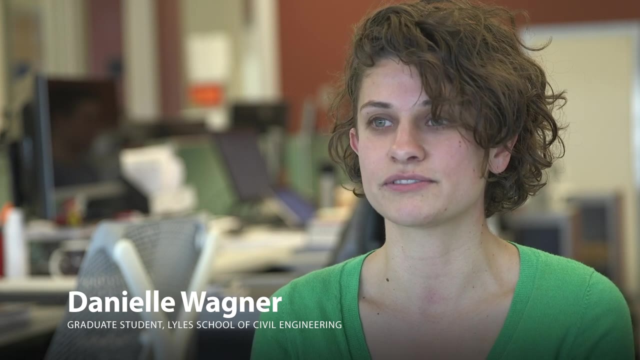 these different locations. We sample the air at that location and then we can see how the building ventilation system affects the dynamics of these indoor air pollutants. There's 12 occupants max at a time. Students have classes, so they come and go, but generally in the afternoons there's a lot of. 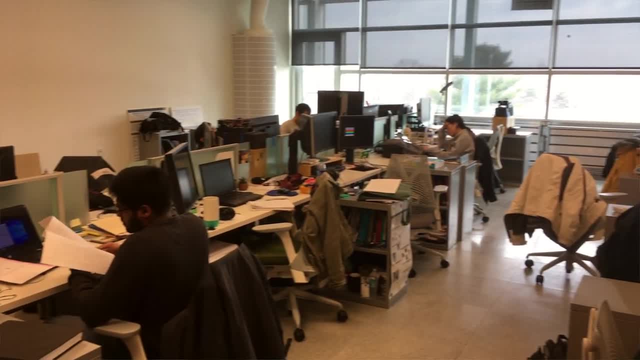 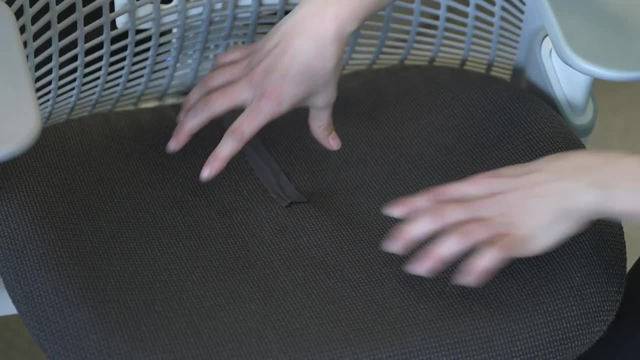 noise. We want to look at how the people affect the air related to the VOCs and the particles, To see the occupancy in each seat. we have thermocouples that measure when people are there, because they sit down and the temperature shoots up and then they stand up and it spikes down. 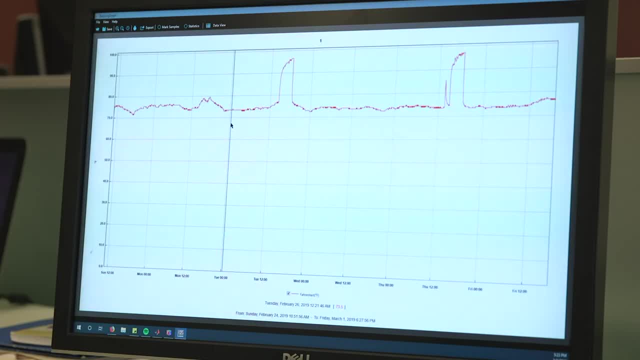 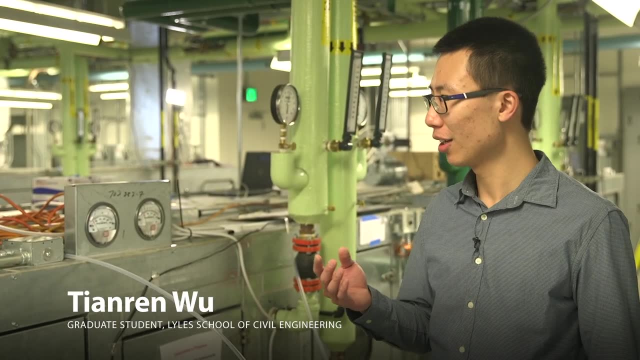 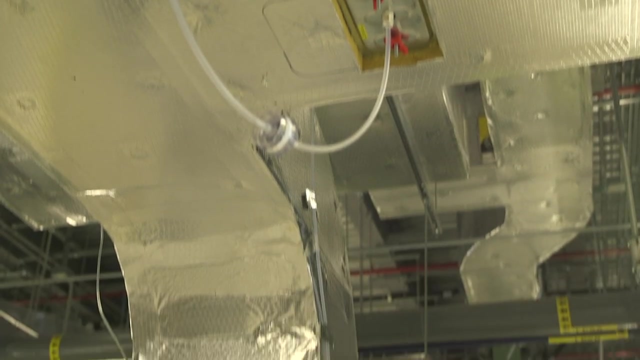 So we can get the spatial map of the room when people are in it. Okay, so we have several aerosol instruments to measure the particular matter: concentration in the air handling units And the return air from the office will mix here and the air goes down First it will pass through. 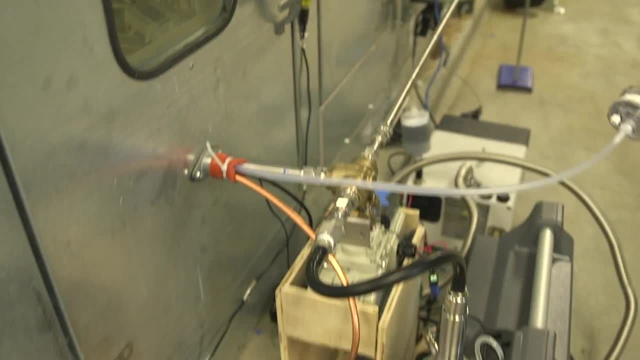 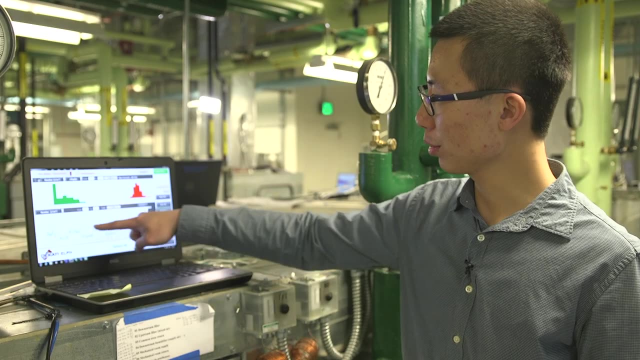 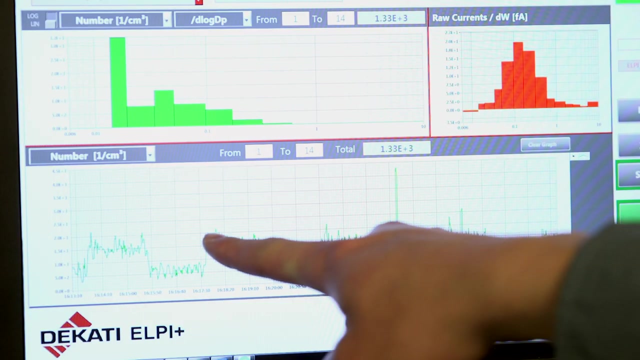 the filter. In the first bank of the chamber we have two instruments to measure the filtration efficiency of particles: upstream and downstream of the filter. By using the data here we can figure out the filtration efficiency of the air handling unit, So here it means the concentration. 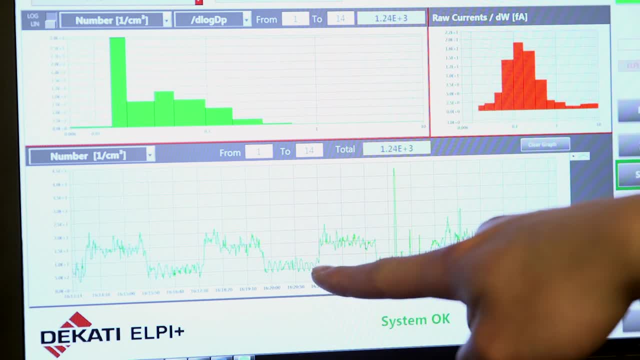 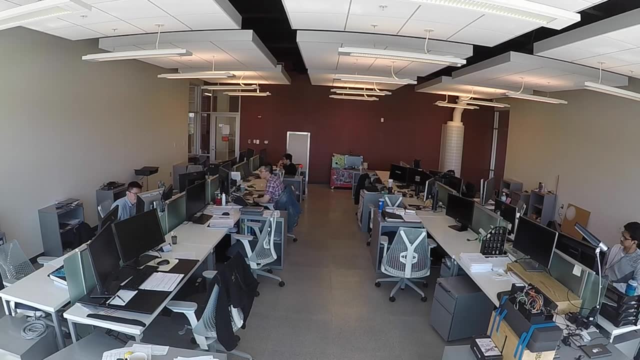 is high, It's from the upstream of the filter and here is the low concentration from the downstream of the filter. So one finding that we have made is that people drive a lot of the chemistry of the indoor environment and we can see that with the different levels of occupancy. 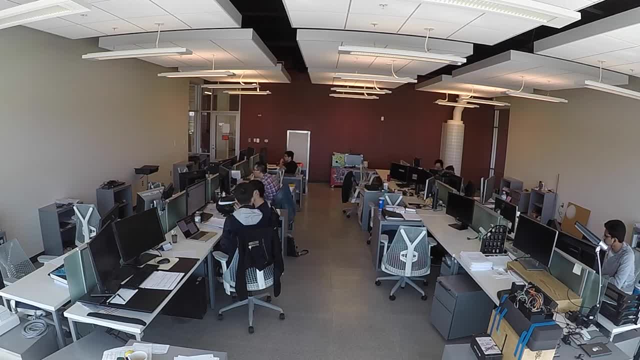 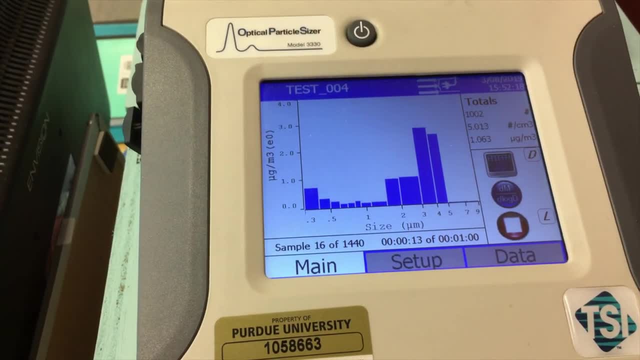 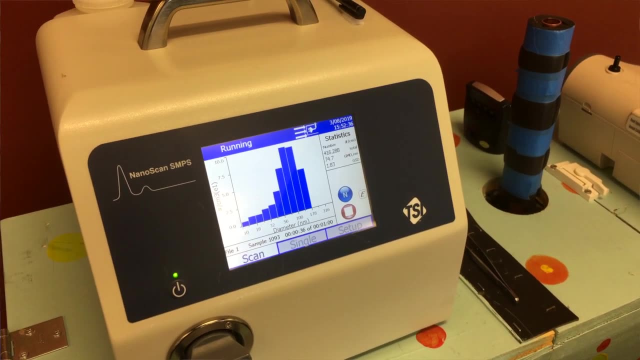 that we're monitoring and then throughout the day the occupancy is constantly changing. we can see how that occupancy drives the amount of indoor air pollutants in the office environment. Another takeaway is that building ventilation can have both a positive effect on indoor air quality and a negative effect. So when we deliver outdoor air to the office space, we can dilute.